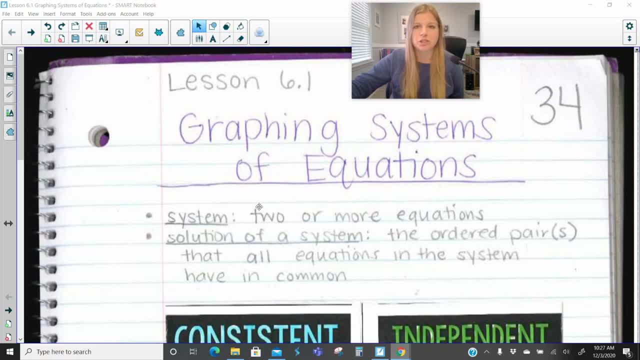 So, first of all, a system means that you're dealing with two or more equations, And right now, in algebra one, we just deal with two equations. Later on, in algebra two, you're going to be dealing with three or more. even So, a solution of a system is the ordered pair. 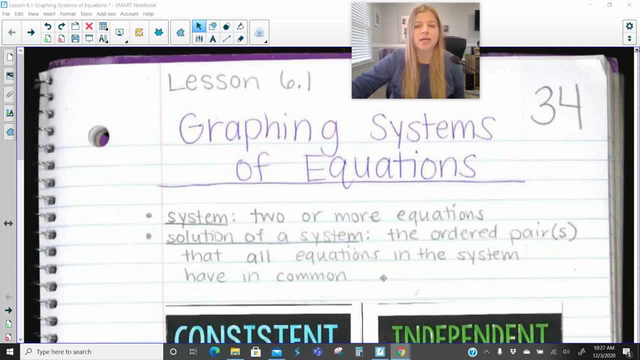 or pairs that all equations in the system have in common. And the way you're going to see two equations actually have an ordered pair in common is if those two lines actually intersect And that intersection is an ordered pair. that is true for both equations in the 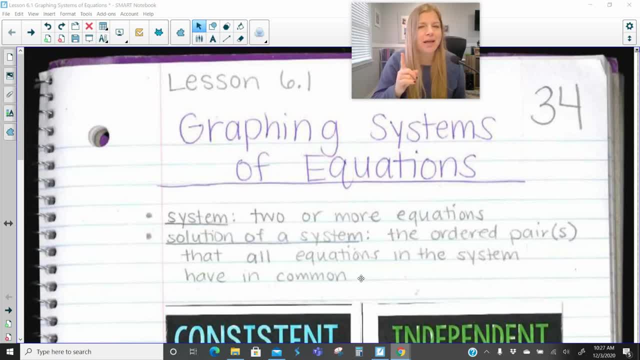 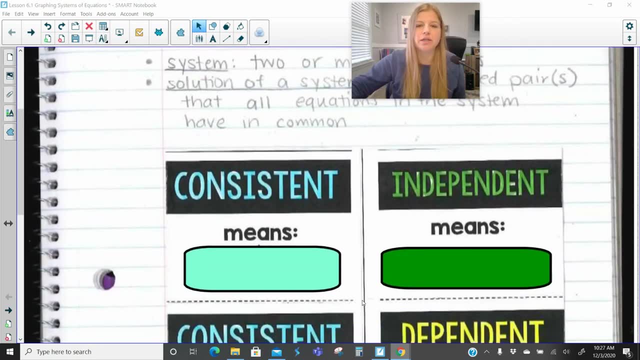 system, But we're going to see. we know that not all lines intersect each other right, So that's going to be something that definitely comes up. We've got some terminology here that we need to make sure we understand. We've got consistent and independent. consistent and dependent. 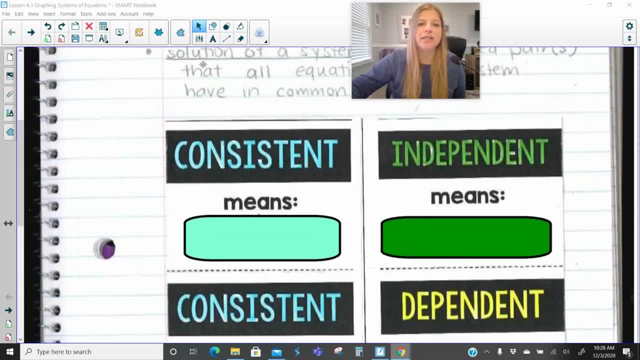 and then just inconsistent. So first of all, if I say the word consistent, consistent is going to mean that there's a solution. So let's say, I go ahead, I give you a system of equations, we solve the system and you find that there is a solution. Well, we then refer to it as consistent. And after: 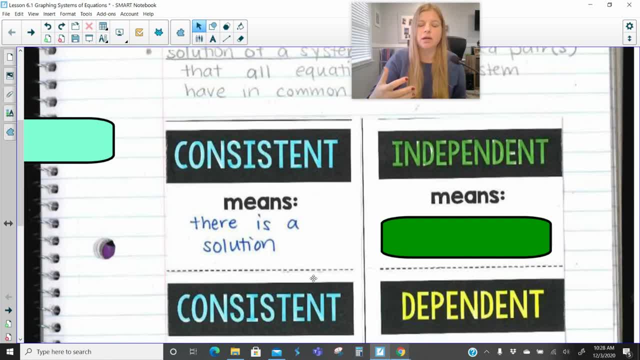 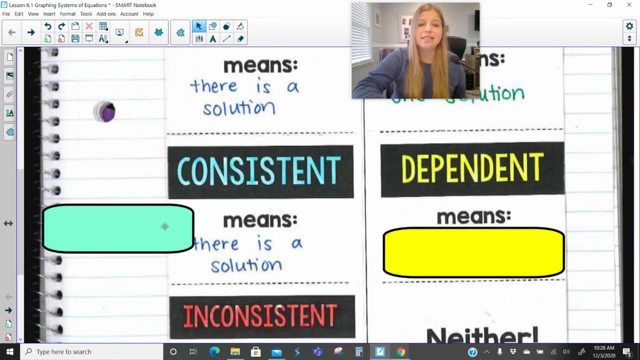 we say it's consistent, we can then talk about how many solutions there are. So we say a system is consistent and independent if there is simply just one solution. We are going to also learn that you can be consistent and independent. Consistent still means there's a solution. 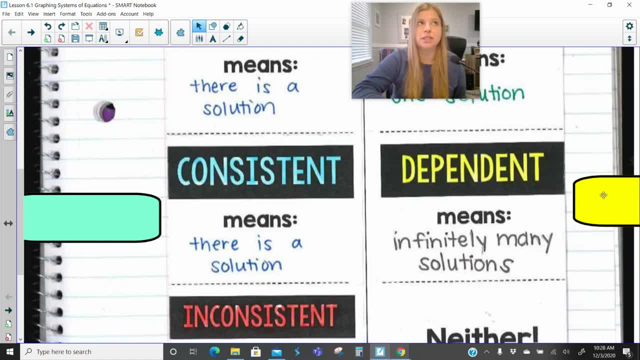 but dependent is going to mean that there's infinitely many solutions. So I'm going to ask that you kind of like think about it like what would that have to mean for those two lines if there's a solution and there's actually infinitely many solutions And we're going to see that in just 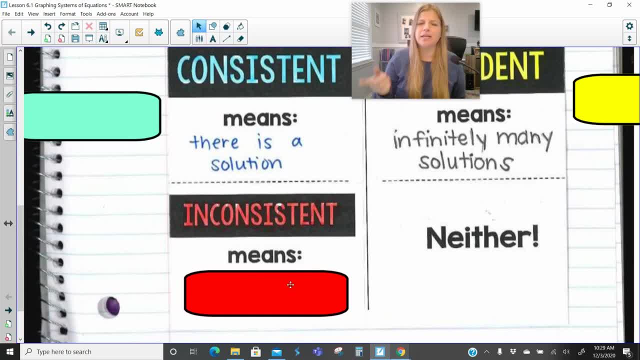 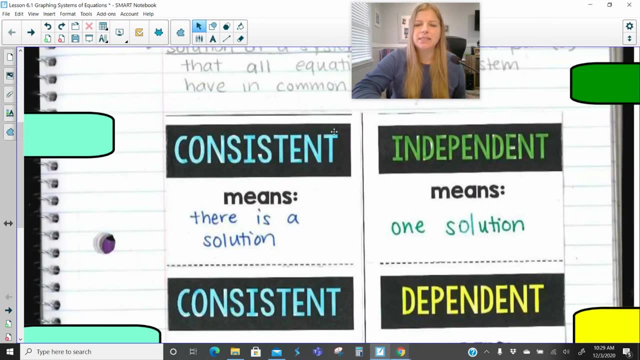 a little bit. And the last one is inconsistent. So think about it: If consistent means there is a solution, then inconsistent means that there is no solution. Okay, so we're going to take a look at two problems of each of these sets. So what consistent and independent looks like, what it? 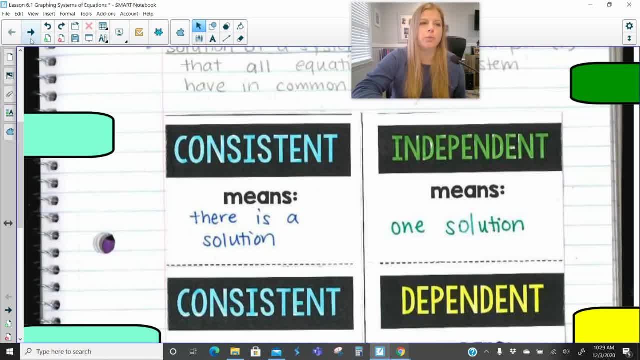 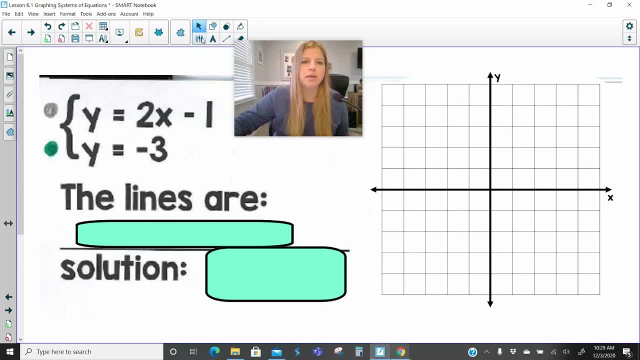 means to have a system, that there is a solution and there's only one solution. So here's our first system. So this first system is: y equals two x minus one, And I have it color coded in gray and green, So I'm just going to probably change it to red, just so it's a little easier to see my graphs. 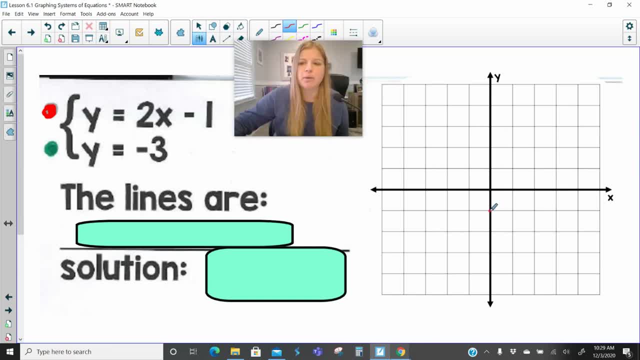 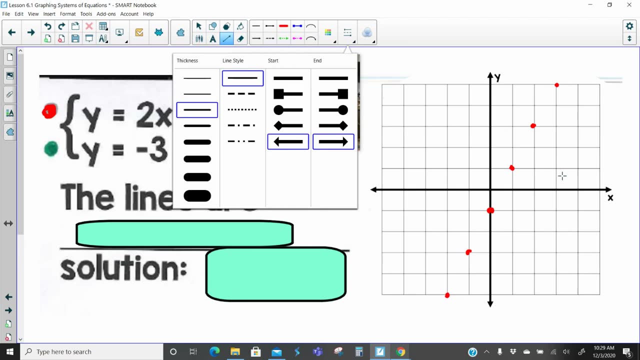 So to graph y equals two x minus one. I know I plot my y intercept at one, my slope at two and my slope at two. Okay, so this is also a little review for our graphing skills. So if you have found that you've been a little rusty at graphing, then this is definitely going to be helpful. for 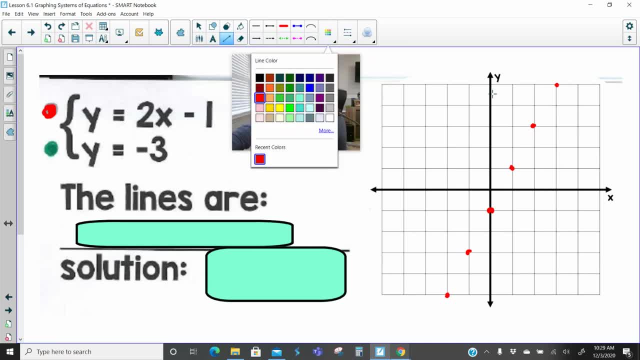 you, And then we're going to go ahead and connect them to make that line. Okay, then in green I'm going to go ahead and graph the second equation. y equals negative three. So we should remember that means on the y axis, at negative three, it is a horizontal line. 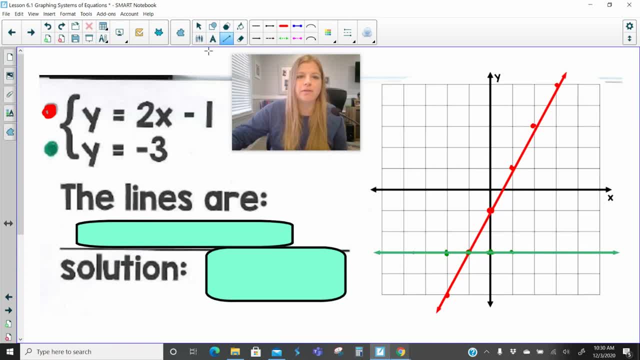 Okay, and now I've graphed my system, And so what we should then see is: well, this system has an intersection. Okay, the lines are definitely intersecting, And the point that they intersect at is actually our solution. So these lines are intersecting. my solution is actually the. 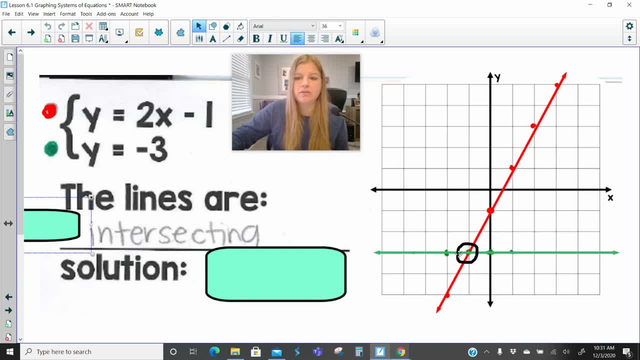 coordinates of this point And you can see, this point is at negative one, negative three, And that is the solution to my system And we're going to go ahead and connect them to my system, And what this actually means- negative one, negative three- is this solution gives you a true statement. 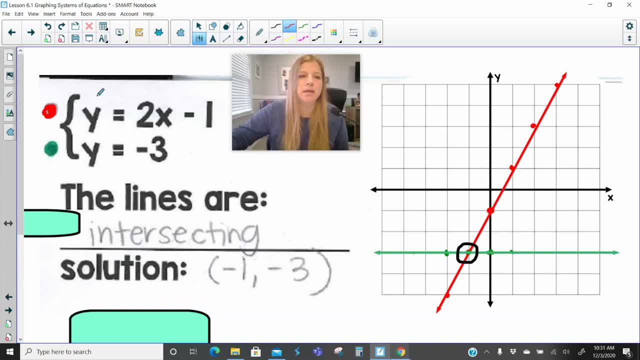 for both equations. So if I went ahead and I plugged in negative three for y and a negative one for x, look what's going to happen two times: negative one is negative two. negative one. negative two minus one is negative three. it gives me a true statement. Here it's just: y equals. 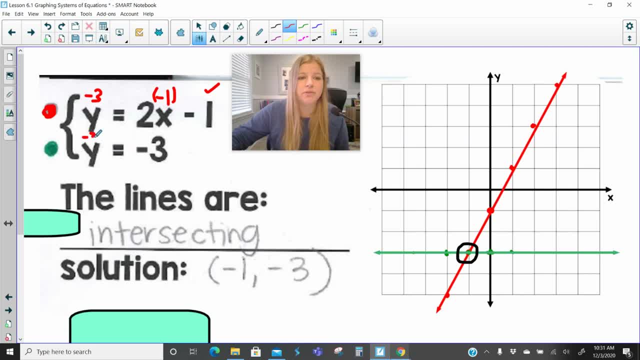 negative three. So that means I just simply plug in my y value of negative three And notice negative three is equal to negative three. So I'm going to go ahead and connect them to my system And it gives me a true statement. This is the only ordered pair that would give me a true statement. 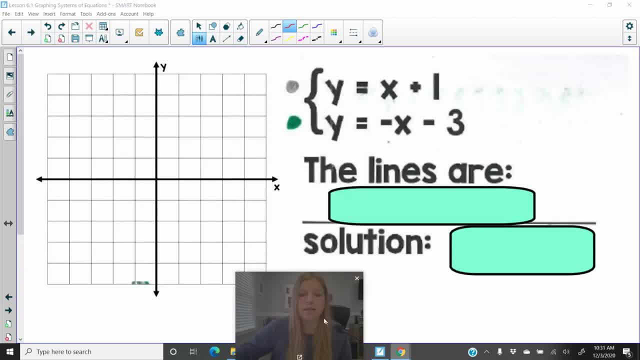 for both of these equations. Let's take a look at this next one. So now I have y equals x plus one. So I'm going to just turn the first one into red. So y, intercept of one, a slope of one. you get the point. Sometimes it can be a little tricky making lines That looks good. So now I'm. 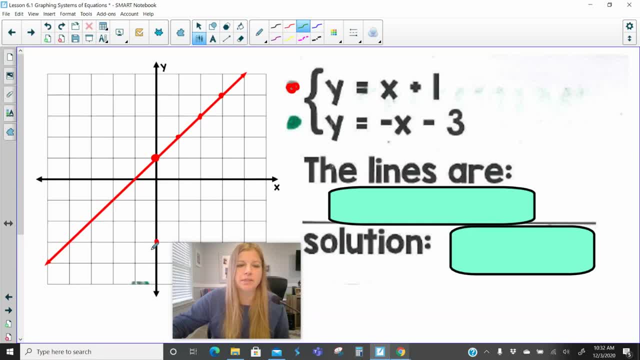 going to go ahead and I'm going to graph my green line. So y equals negative x minus three. So I have a y intercept here at negative three, a slope of negative one. You can already see that these two lines are definitely intersecting each other. 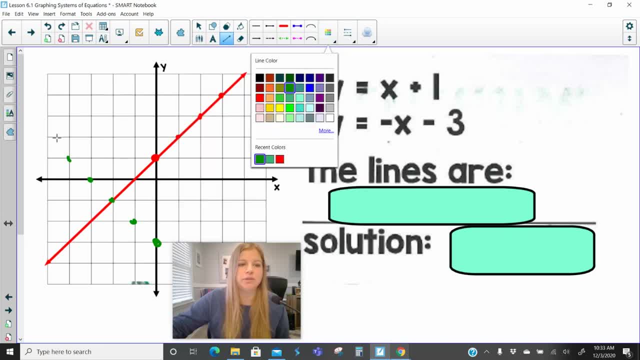 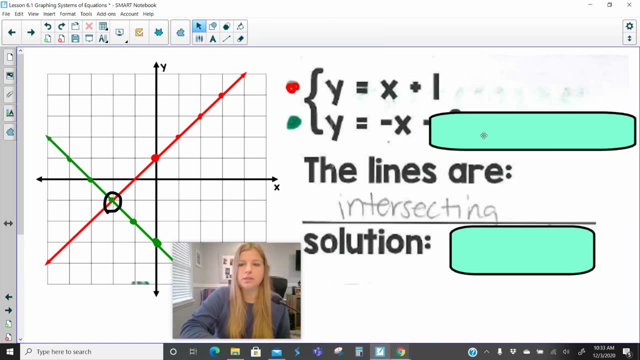 which is fantastic. I'm going to change my line to green point to graph. this line goes right through my screen box. here I can clearly see that these two graphs are intersecting each other And the coordinates of that intersection are my solution. So these lines are intersecting. 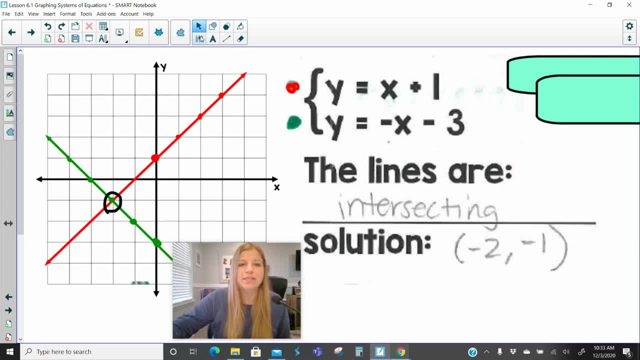 the solution is negative 2, negative 1.. This is what consistent and independent looks like, guys. If I was to substitute negative 2 and negative 1 in here, so it's y is negative 1,, x is negative 2, and notice, negative 2 plus 1 is negative 1.. It's a true statement. If I go ahead here, 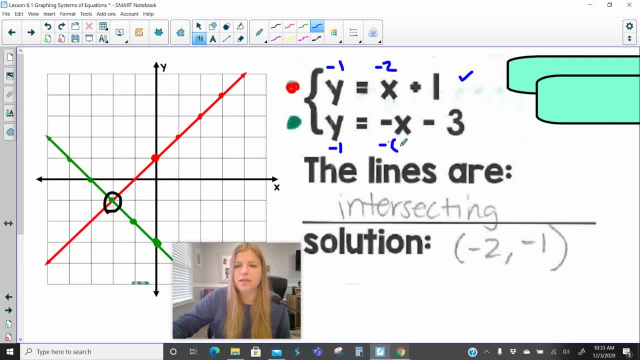 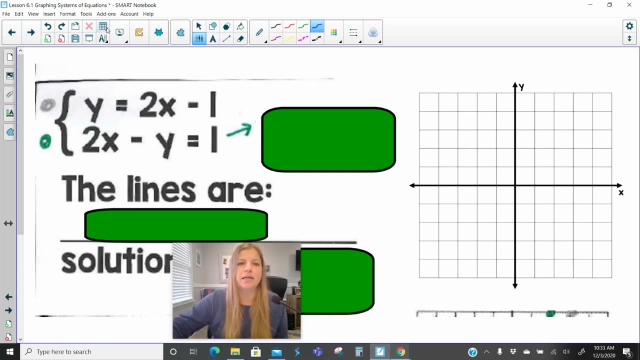 and I plug in a negative 1 for y, and this would be negative negative 2 minus 3,, which really means positive 2 minus 3,, which is definitely negative 1, and that gives us our true statements. Now the next two problems are going to be consistent and dependent. 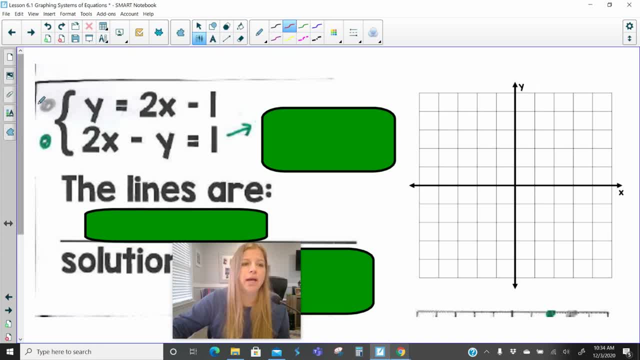 which means all real solutions. So if I go ahead and I graph this first equation, y equals 2x minus 1, I have a y-intercept at negative 1, a slope of 2.. This is just like the first graph that we did before. I'm going to graph my line, Then I'm going to switch over to 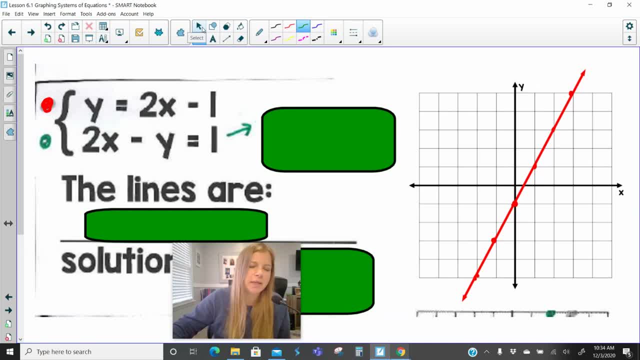 green. Now I should notice also here too, guys, 2x minus 2 is negative 1.. So if I go ahead and I graph this first equation: y equals 2x minus y equals 1, I have a y-intercept. 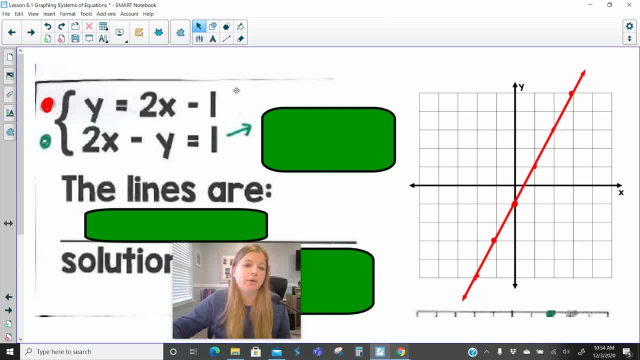 at negative 1.. I can find my intercepts and graph, or I could rearrange that equation into slope-intercept form, which may also help me graph it. So I would need to subtract 2x on both sides and then multiply the entire equation by negative 1.. So I end up getting 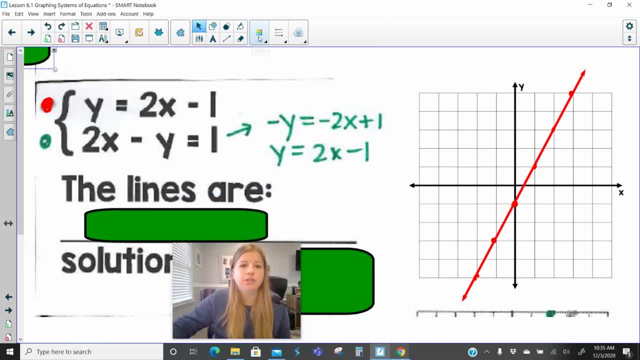 an equation in slope-intercept form, And then I can go ahead and actually graph this equation. So my y-intercept in this equation is negative, 1. My slope is 2.. And then I can go ahead and do. what do we notice? This equation is identical to this equation. And if I go, 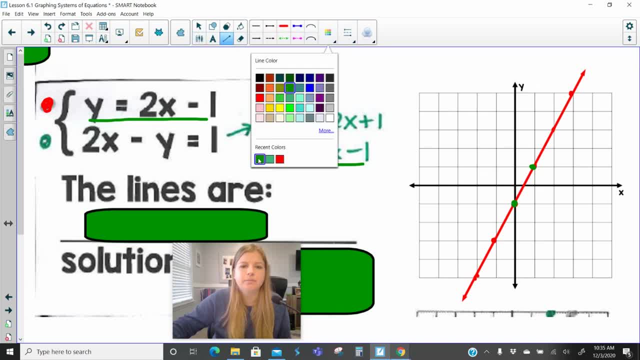 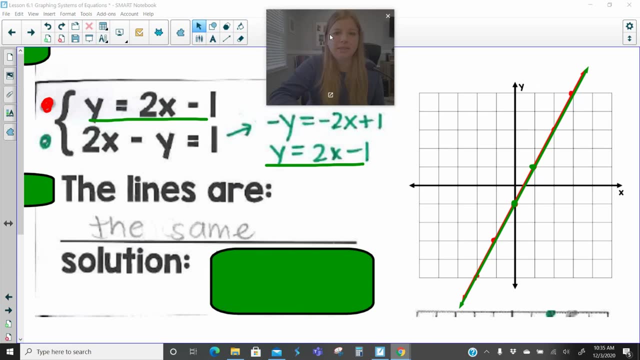 ahead and I make a line of that equation. obviously the lines are going to overlap each other, So every point on the red line corresponds with every point on the green line, And so these lines are exactly the same, which means our solution is infinitely many. So any point. 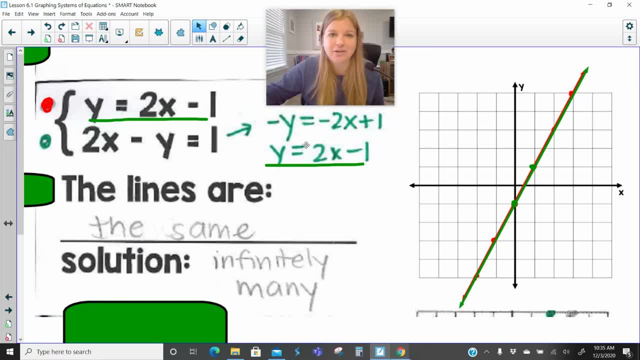 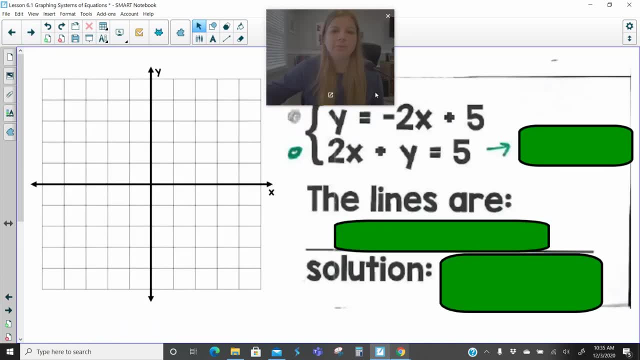 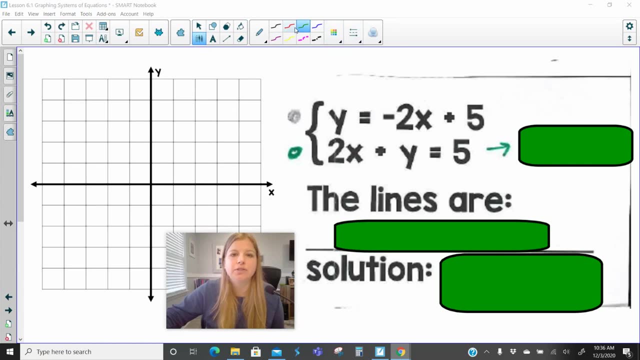 obviously. So one equation here is going to be identical. if I plug it in to the other equation, They're all going to work. You have infinitely many solutions. So this next problem you're going to see follows that same idea. I have my first graph here. y equals negative 2x plus 5.. I'm 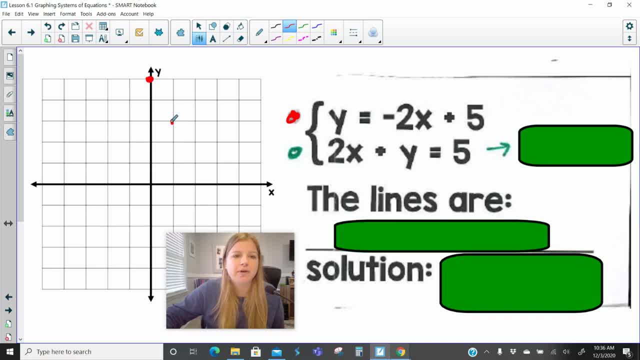 going to put that in red. Okay, so y-intercept of 5, a slope of negative 2, we get the point. And then I'm going to put that in red, And then I'm going to put that in red, And then. 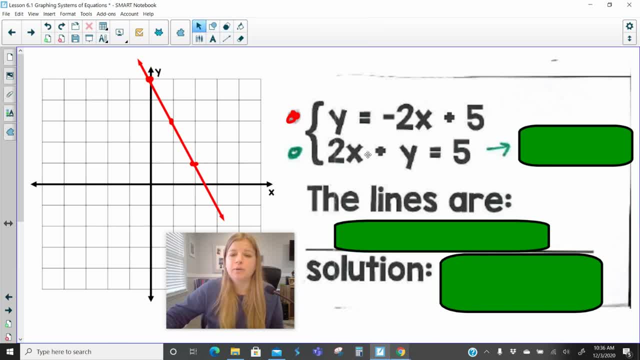 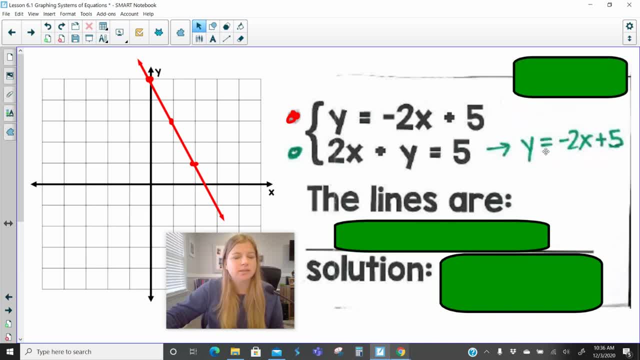 intercept form. I would subtract 2x And what I'll notice is: this equation is identical to the other equation. I think you get the point. for this I don't need to graph the green line over the red line, And that is again infinitely many. So when you have lines, 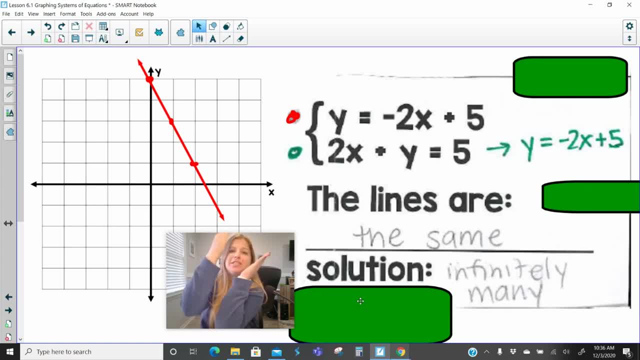 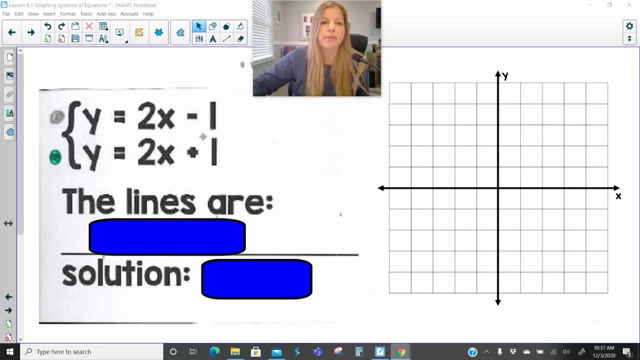 that intersect. there is one solution If they are actually the exact same line. if two equations are the exact same line, that is when they are infinitely many, It's infinitely many solutions. Okay, let's take a look at this one now. So y equals 2x. 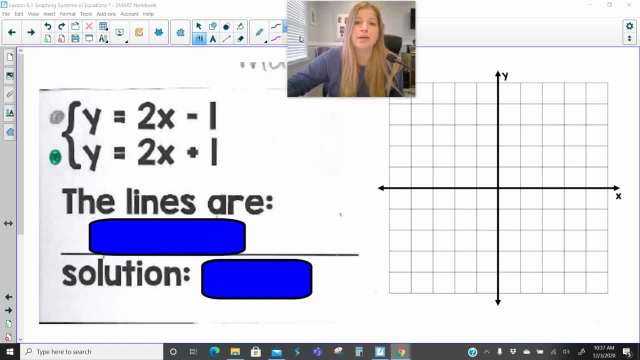 minus 1, and y equals 2x plus 1.. Now, hopefully, I could only hope that you learned a very important lesson recently where you learned about slopes And we can see that these two equations have the same slope, So hopefully you're already thinking about something that. 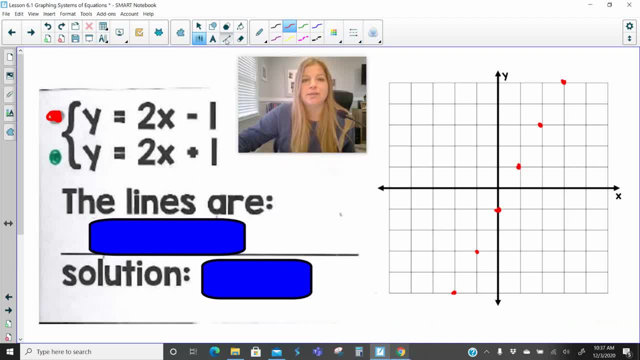 you know is going to happen with these lines. Okay, so I'm going to switch over and I'm going to graph my line through those points. I'm going to switch over to green and graph my second: a y-intercept of 1, a slope of 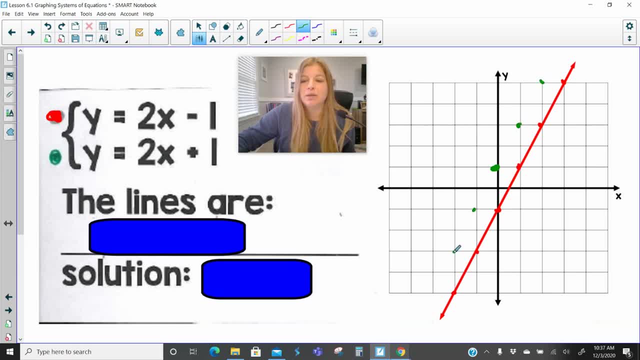 2. Hopefully we see that these lines are definitely parallel And we could tell that they were parallel before we even graphed them because, remember, parallel lines have the same slope. So if I go ahead and I graph these lines and I see they're clearly parallel,